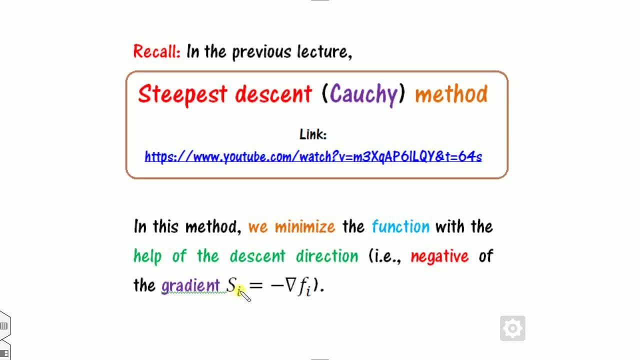 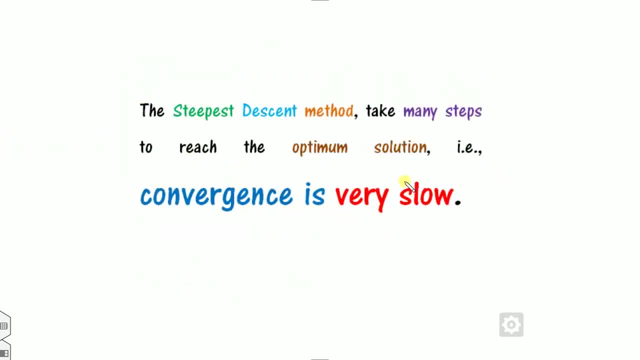 with the negative of the gradient called as the SI, my certain direction. But once we see that, when we solve any kind of the optimization problem, unconstrained optimization problem, with the help of this steepest descent, we will see that the convergence is very slow, or you can see that there are 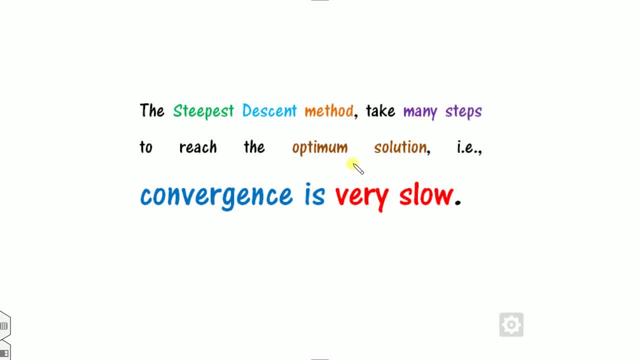 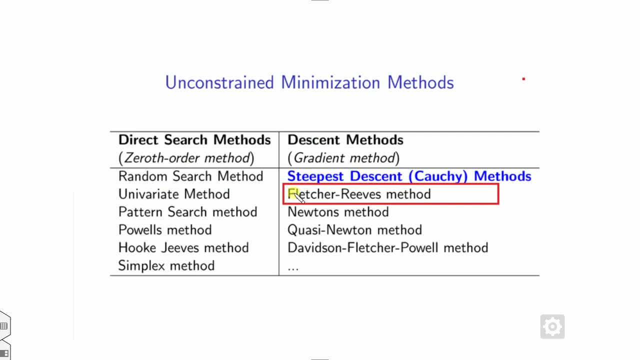 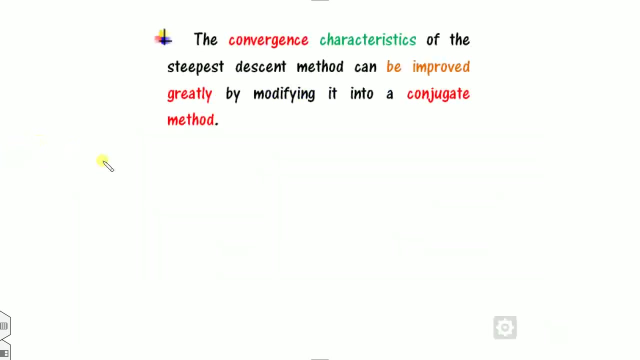 they takes many steps to reach the optimal solution. So how to increase the convergence of this unconstrained optimization method? So, in order to handle this, we will try to learn the second method that is called as the Fletcher-Reeves method. What did this Fletcher-Reeves method is that? the basic feature is that the convergence characteristics of the steepest descent method is improved by modifying into the conjugate method. Now here is what is the conjugate method? So what is that? in the conjugate methods, the conjugate directions involve the use of the gradient. So what is the conjugate direction? So any 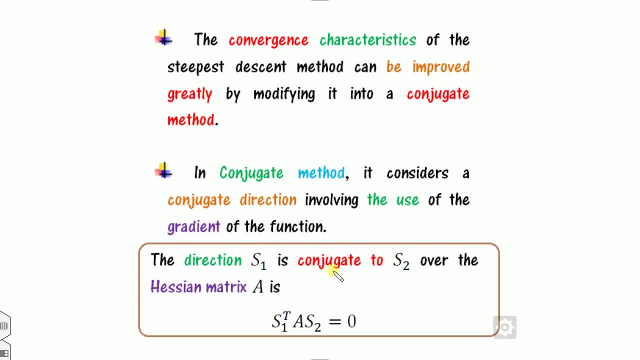 any direction s is conjugate to the s and you know that. what is the meaning of the conjugate? that is the perpendicular in the layman language there, But here the direction s1,. if I say this is my minimum and if I say this is my direction and this is my gradient- sorry, this is my gradient, Okay, so this is my gradient of that. So if you find the direction s1, okay, so if you take, this is my 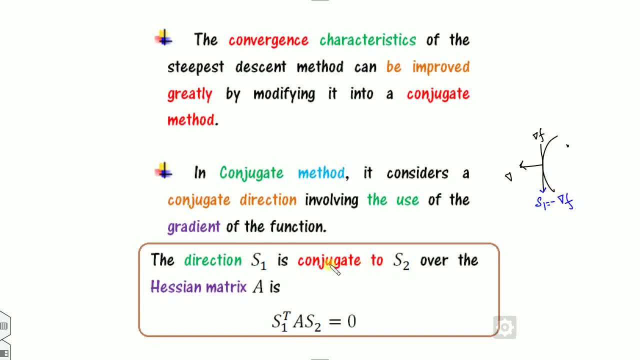 s1,, which is nothing but minus of the gradient and direction, is conjugate to the next direction if this property holds. So if I say this is, say, my s2.. So this is my perpendicular here is not be directly perpendicular here. It is with respect to the Hessian matrix. if this conditions hold, So any two direction are said to be conjugate. if this direction holds, So for any minimization problem, this conjugate. 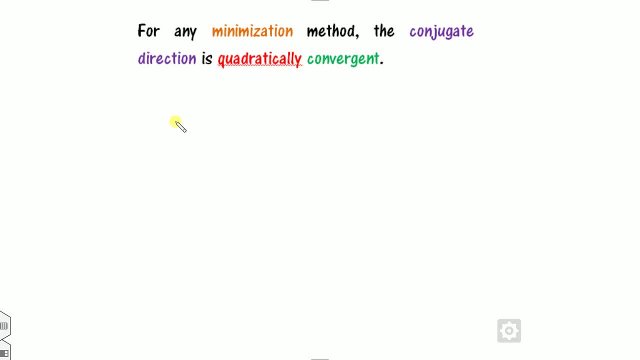 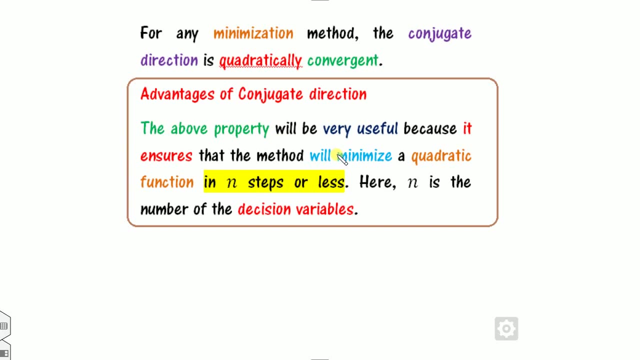 direction is the quadratic convergence. So what is the advantages of this quadratic convergence? that it advantage is that whenever we are trying to solve any quadratic optimization problem, then the convergence will be take at the most and steps. What is the end step is and is the number of the decision variables. means if I say my this function is there, So how many decision variables are there to x1 and x2.. In this example you look at that, how many? 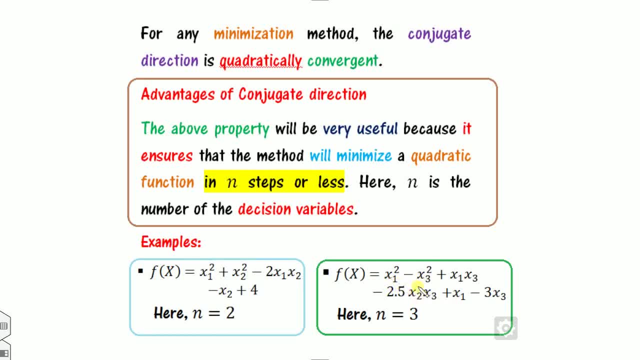 direction. decision variables are three. so it means when we trying to solve this problem with the help of the conjugate gradient method, then it take maximum three steps are there and after the three steps, or after the three steps means after the three iteration, at the third iteration, conjugate. 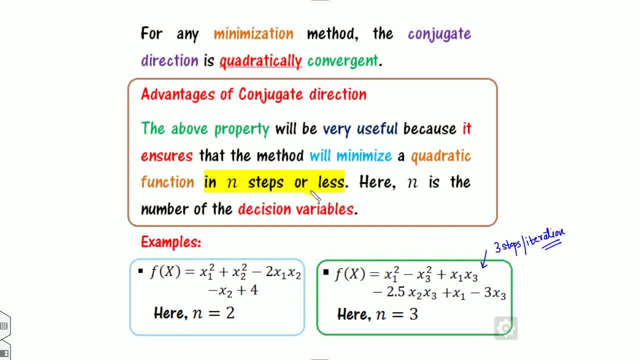 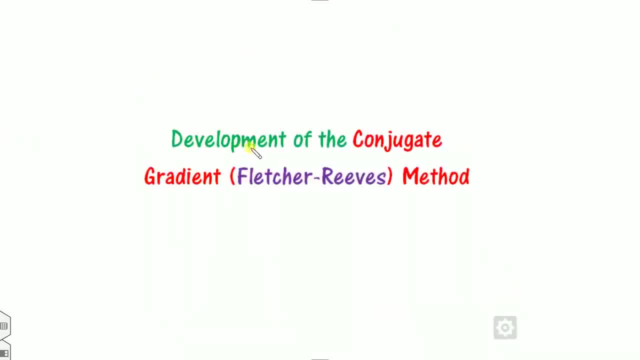 direction method converges to the optimal one or it can be less than so. it can be converges in the second step or initially at the first step, also. so how it works that. so what is the development of the conjugate gradient, how it develops that. so what is that initially? i just consider the 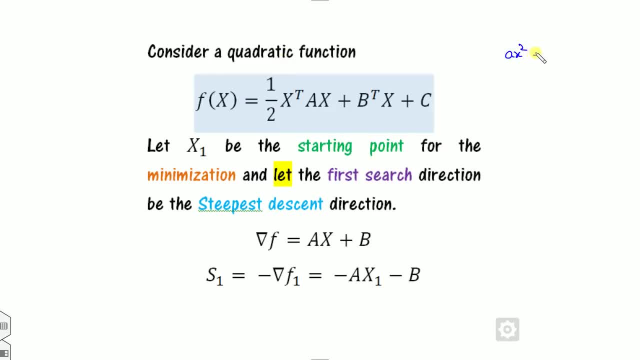 quadratic function. you know that in general the quadratic function is ax square plus bx plus c. this is in terms of the real numbers, are there? so if i represent in terms of the matrix, so this can be written as x transpose ax. since it is a matrix, so this is bx plus c, is there? 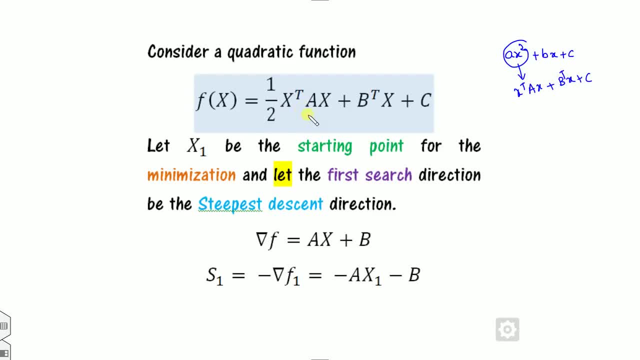 so i just half represent perdon in order to reduce this. simplification is there. So assume that x1 is my starting point and the first direction is used by the steepest descent. What is the meaning of that? That is based on the previous lecture. So what is the gradient of this? So you know that. 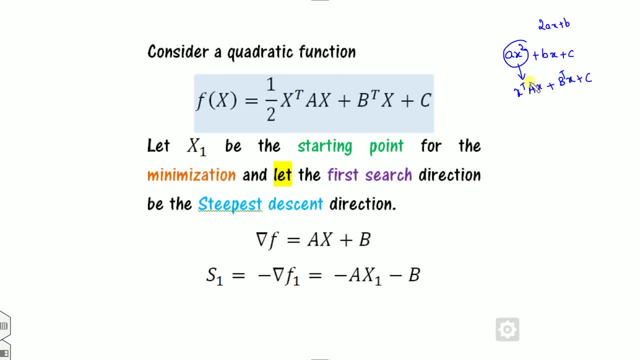 what is the gradient of this? is 2ax plus b. So if I use the half of here, so what is the gradient of this? is nothing but ax plus b. So look at that and look at that. this is my steepest descent direction. First one is used: the s1 is nothing but the minus of 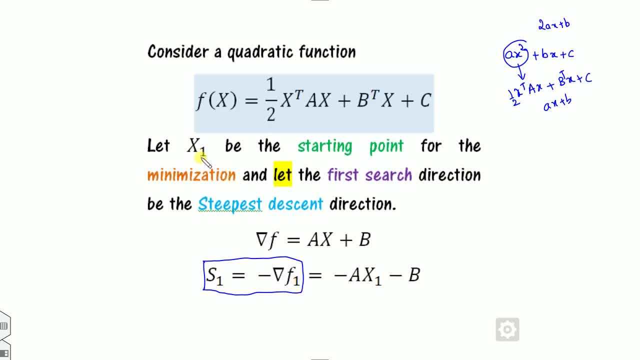 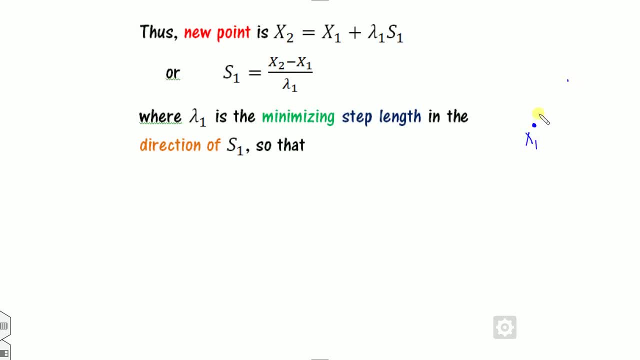 gradient. So this is So 1 represent for my x1.. Now, so the new point. it means you start from here. This is my x1.. You reach at this point. This is x2, with some length. This is my lambda 1, and this direction is called as the s1.. So what is that You can? 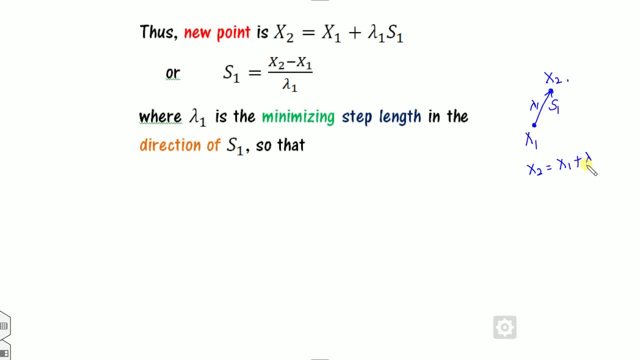 calculate this as x1.. Plus what is the magnitude and there So you can find the value of this where lambda is calculated as the minimization of the direction. So if it is minimizing that, you can easily find that s1 transpose of the gradient at this point. So since what is my gradient? 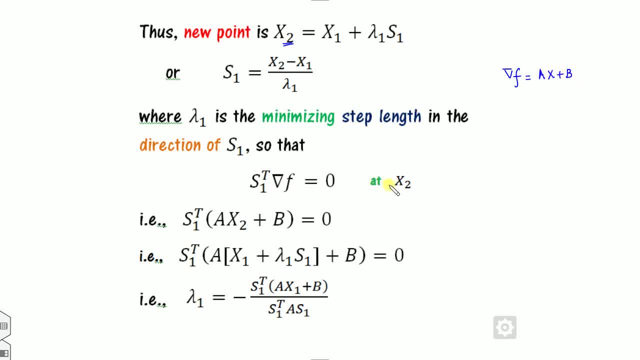 Gradient is nothing but the ax plus b, So at x2. what is the meaning of the at x2?? This is nothing but the ax2 plus b, So I just substitute value here. What is the value of the x2? It's x1 plus this, So 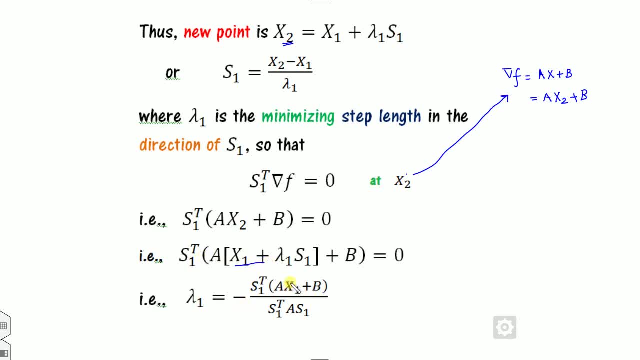 I just open the bracket and I just calculate here and look at that. what is the value of the x plus b? So if I this? so what is the value of the ax 1 plus b? This is nothing but the gradient at the point x1.. So this is nothing but my this one. And since what? 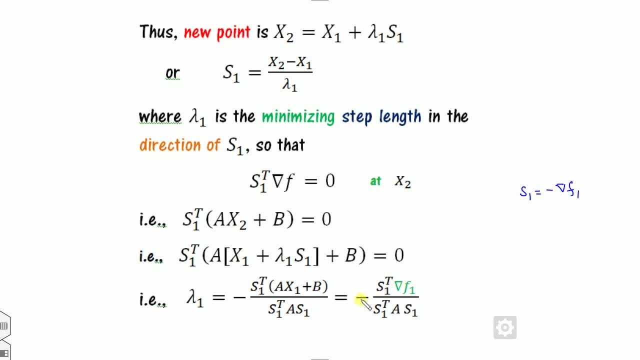 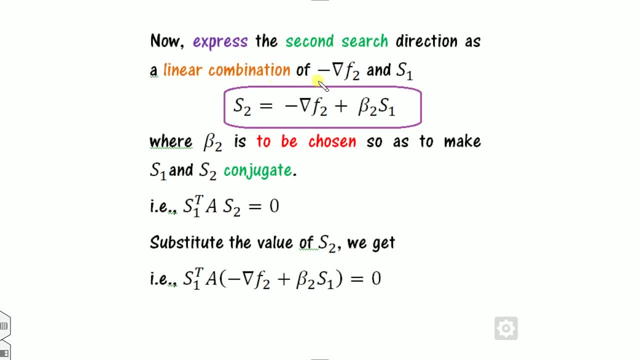 is my. s1 is nothing, but here 全 substitute root value of this. so you will get this number. so s1 is nothing but the minus minus plus. so the lambda is here now. now, this is the first search direction. so second search direction is written as the linear combination of gradient and this search direction, if you remember the. 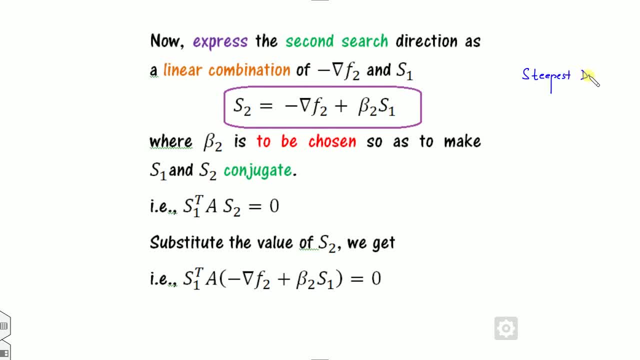 steepest descent method. so what we do in the steepest descent method is: what is my s2 is simply here. this is my steepest descent method. now, in the conjugate gradient we have to add the linear combination of the previous one. this is the s1 direction, the previous one. so how you choose. 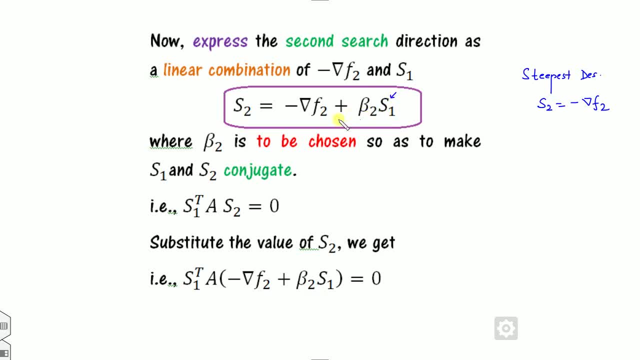 this beta 2. so this beta 2 is chosen in such a way that s2 and s1 are conjugate. so what is the direction? is s1 transpose a s2? is 0 is the definition of the conjugate. now, substitute the value of the s2 here. you will get this now after opening the bracket. 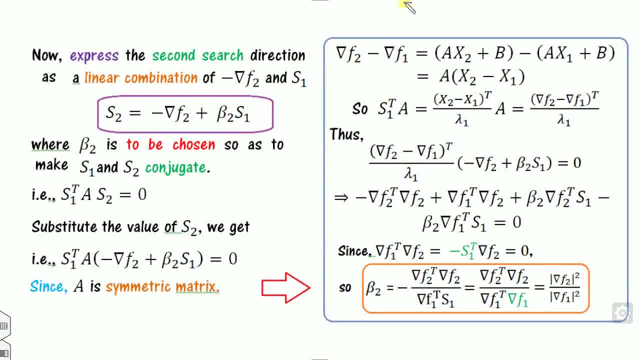 you will simplify that, you will get. look at that. what is my again. what is the gradient is ax plus b. so what is the gradient at x2 minus gradient at x1 is here and look at that. the first value this: what is the value of the s1? we have calculated the previous slide: x2 minus x1. 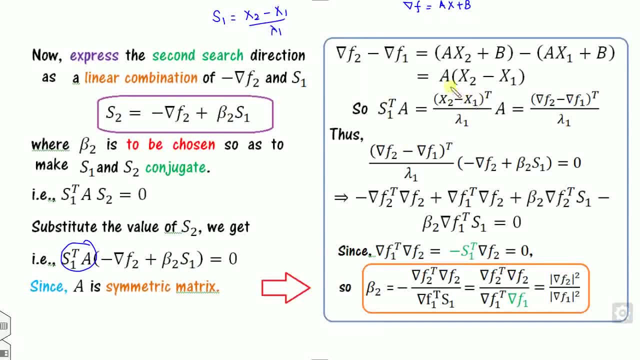 upon lambda 1, so i just substitute here. so look at that, the value of here and the value of here. so this is so. what is that? this is a transpose, so this is here. and since a is a symmetric matrix, so what is the meaning of this? metric is a transpose, is nothing but the a. so i just represent here. 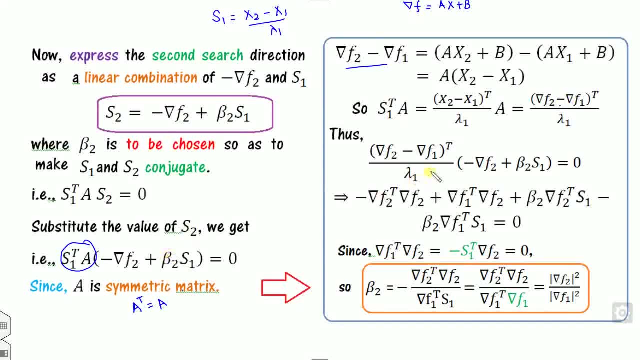 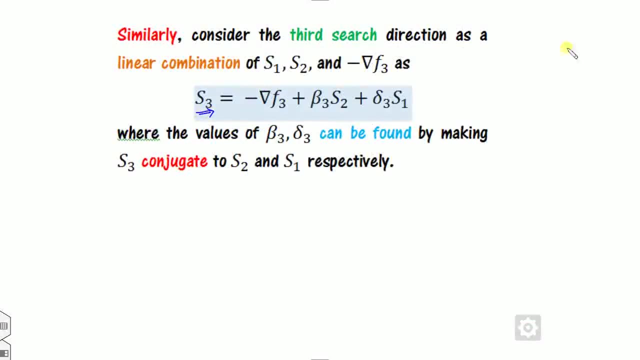 now substitute this value in this equation, you will get this. and after, simplify, you will get this. so remember this last line: beta 2, that is, the value of this, is nothing but magnitude of the gradient at the second point divided by the gradient x, and you will get this, this one. so, similarly, you can find the direction at. s3 is now, since we have 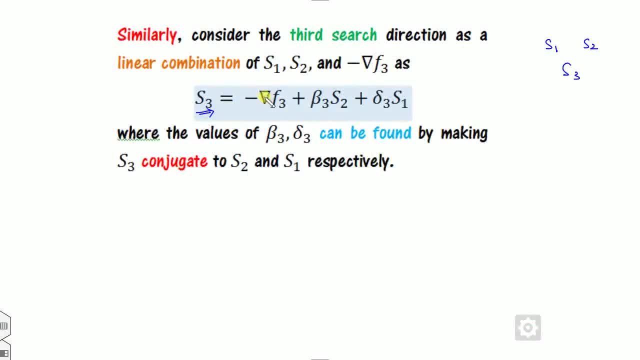 s1 and s2, so we can write this s3 as minus of the gradient, this linear combination with respect to this and linear combination with respect to this. okay, and how you choose the beta 3 and delta 3 by the same property, beta 3 can be chosen in such a way that s3 and s2 are all conjugate to each other. 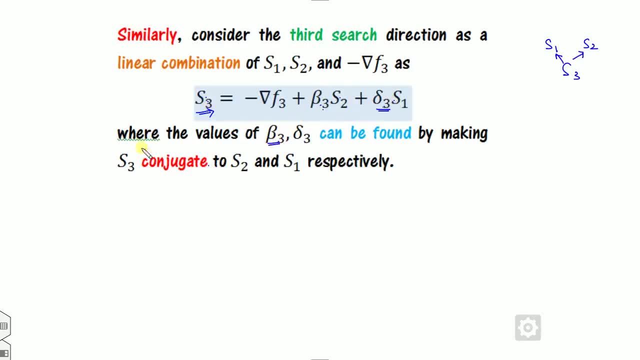 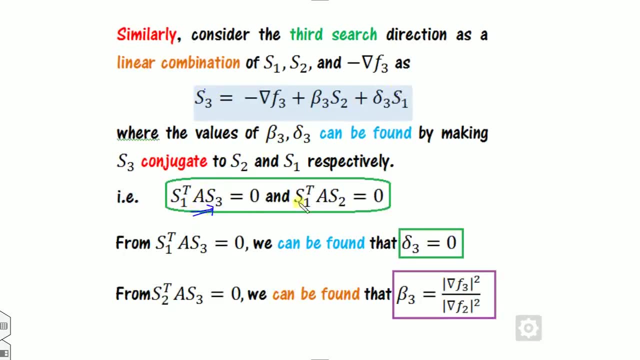 delta 3 is calculated as s3 and s1. so what is the meaning is that when you say s3 and s1 are conjugate, so it means this property holds and this property hold for the beta 3. so when you solve this property, when you substitute s3 here and use the previous calculation, you will get the delta 3: 0. 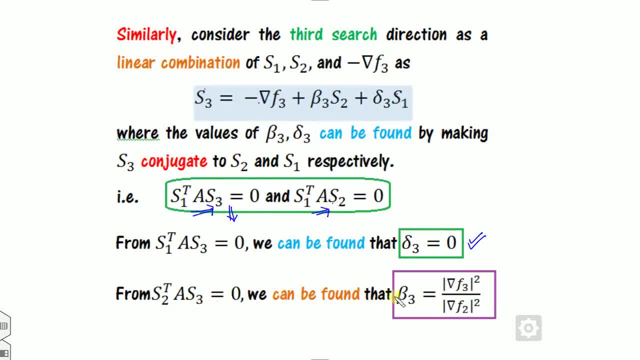 when you try to solve this with the previous case, then you will get this okay. so look at, the beta 3 is nothing but the this and in the previous slide you will see that this is my value of the beta 2. and look at that: this 2, index 2 and. 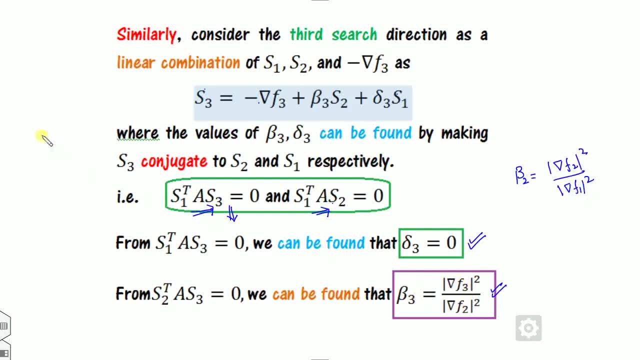 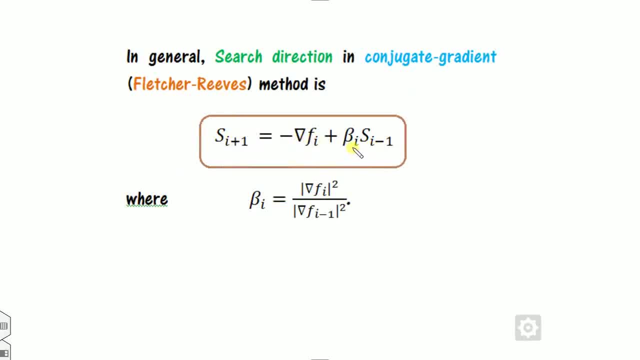 this is 1, this is 3, this is 3 and 2. so in general, we can see that s i plus 1 is nothing but this linear combination of this one and this beta is nothing but this i and so on. so, with the help of 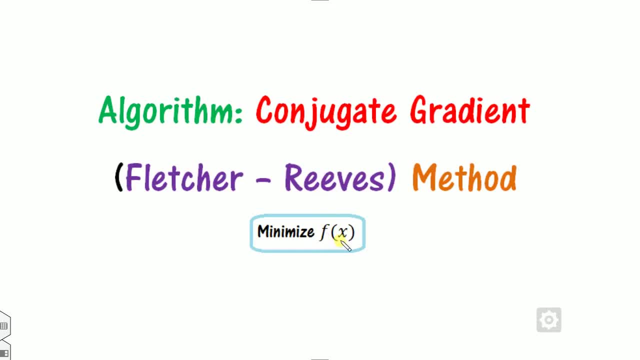 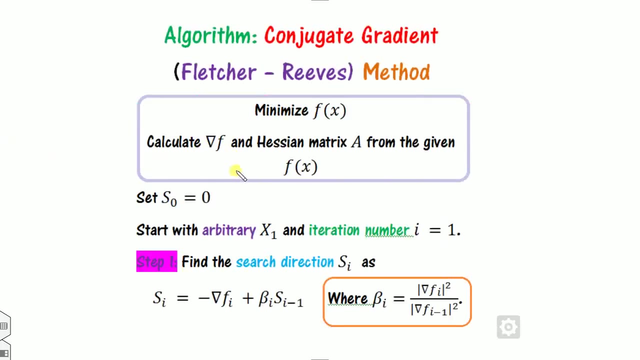 this theory, we can algorithm, design the algorithm for minimizing the effects. remember that if my objective function is my objective function, then the objective function is my objective function. so you need to firstly convert into the minimization by using this rule minus of this, and after that we will solve this minimization again. so what is that? you can firstly calculate the gradient. 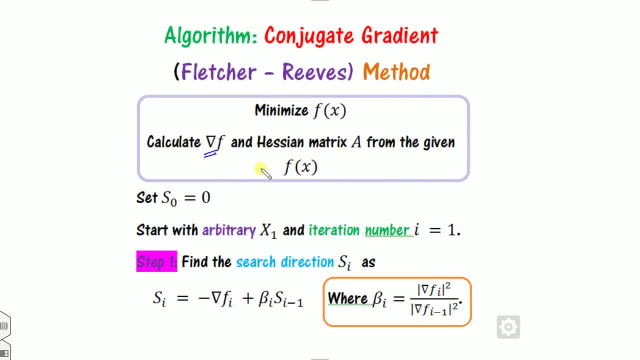 you can initially calculate the hessian matrix and since we start the equation 1, so i then can set the s 0, that is a 0 search direction, at 0. so now the search direction s- i is ruling at this- where beta is this? so what are the steps? are there? so, first step, you can use that. this is the three step rule. 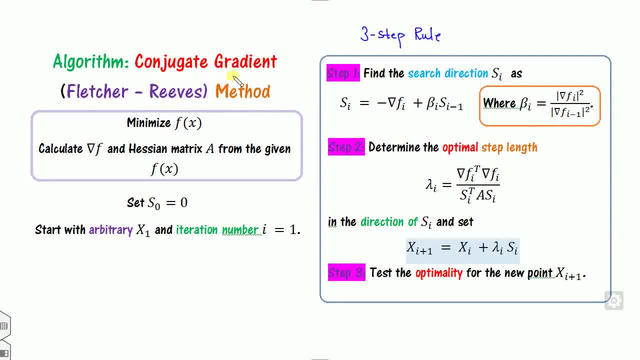 always remember the three step rule for solving the conjugate gradient methods for any unconstrained optimization problem. first direction is first step is here. you can calculate beta so we can explain the numerical example also, while this rest are similar as that of the steepest descent. 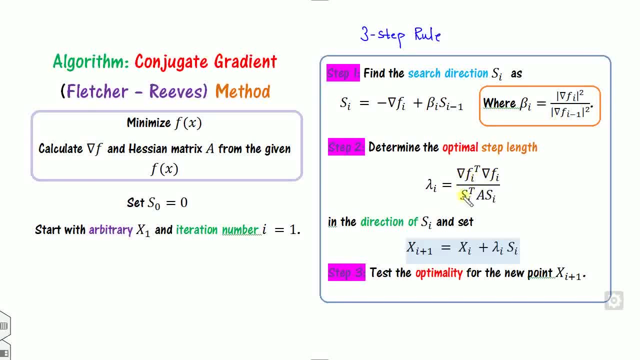 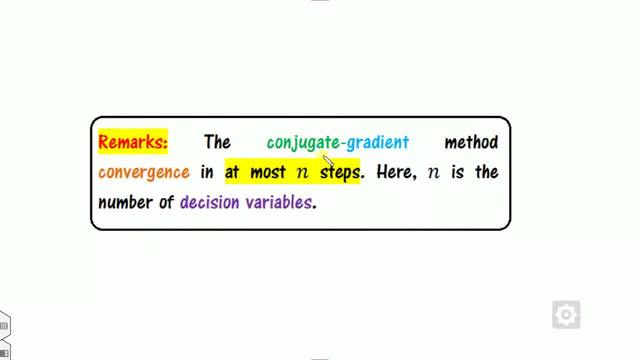 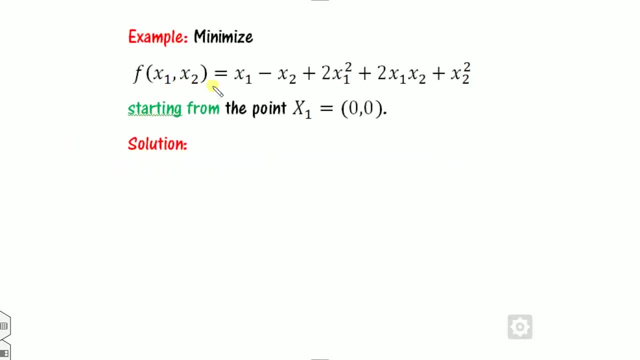 in the steepest descent. we also use this one gradient divided by this check whether the optimates or not. and the more most beautiful advantage, that the conjugate gradient method converges at the most. and steps are there. so look at this numerical example. so consider this minimization problem. so look at that. 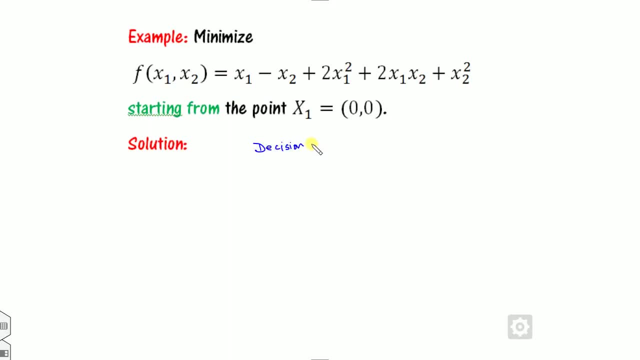 how many decision variables are there? so what is the decision variables are there. this is my x 1 and x 2. so that is now: n is 2. it means when you solve this by conjugate gradient method. so how many steps are there? how many equations are there? that is maximum. 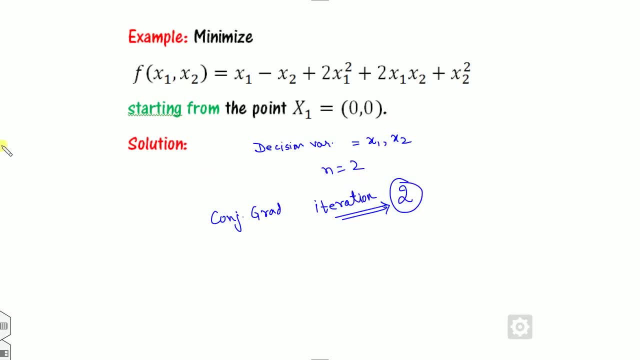 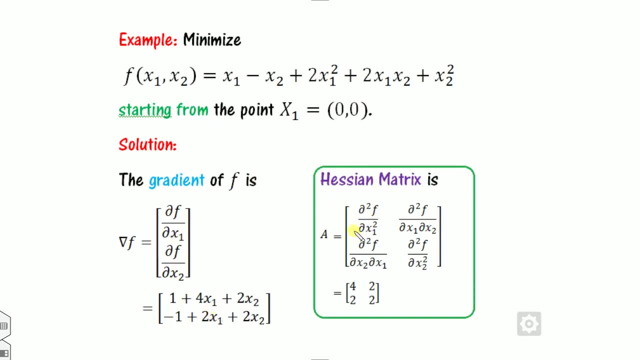 to maximum 2. okay, so now, firstly, we can calculate the gradient of this. so, gradient is this one. you can say how you find the hazen matrix, since it is a decision variable is 2, so this is nothing but my 2 cross 2. always remember my. this is the hazen matrix a 11. this is the 2 cross 2 journal matrix. what is 1- 1 is that is derivative 2 times with respect to x1 a- 1. 2 means derivative 2 times with respect to x 1 a. 1. 2 means derivative 2 times with respect to x1 e 1. 2 means deriving this derivative. 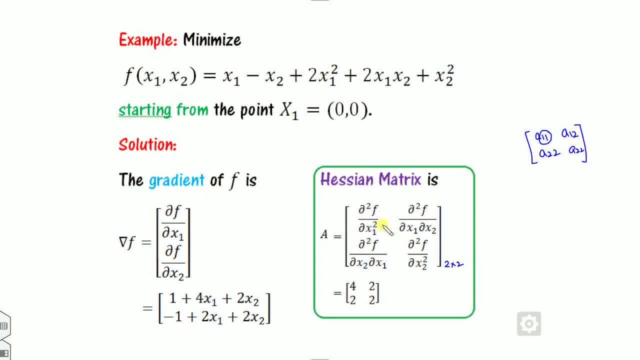 name p 1, that is magnificent. then the signal to بن brown shouldn't be another matrix. this is the two, non, non, once to theforger mode. p one is two. now what is the derivative two? and outcome is in Throwback: a 1, 2 means derivative of this f, firstly with respect to x 1 and then with respect to x 2. 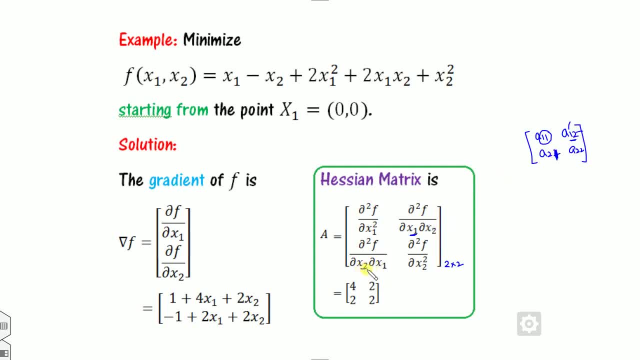 here is sorry, it's a 2- 1, so firstly with 2 and then 1 and so on. so if you derivative this twice with respect to x- 1, you will get 4, 2, 2 and so on. now start with the three step rule, are there? 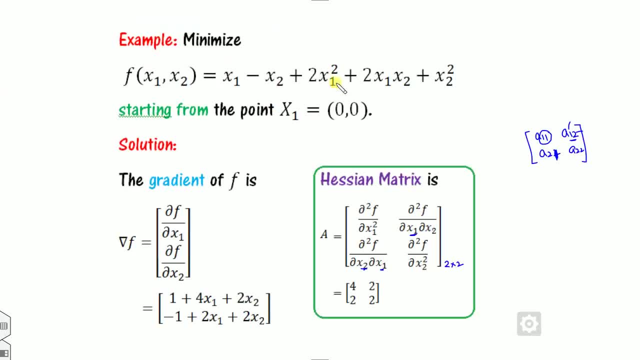 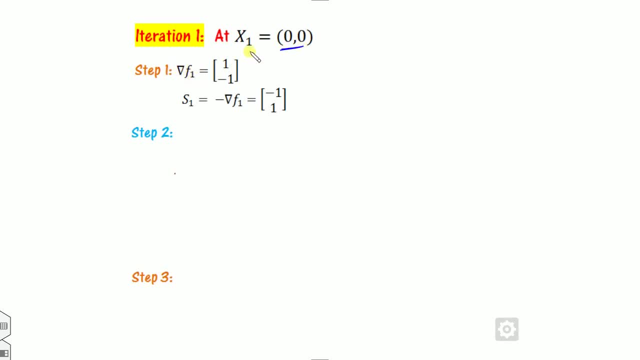 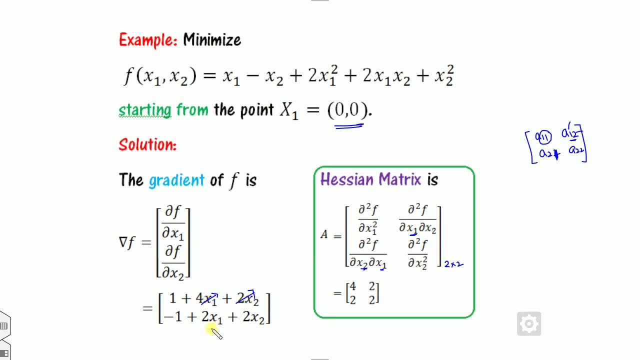 first point is iteration. initially is given to be 0, 0, so this is given. firstly, find the gradient. gradient at the point 0, 0. so we have find the gradient here. so what is the value? at 0, 0, so this becomes 0, this 0, this 0, and so get 1 and minus 1. so 1 and minus 1. so what is the value? 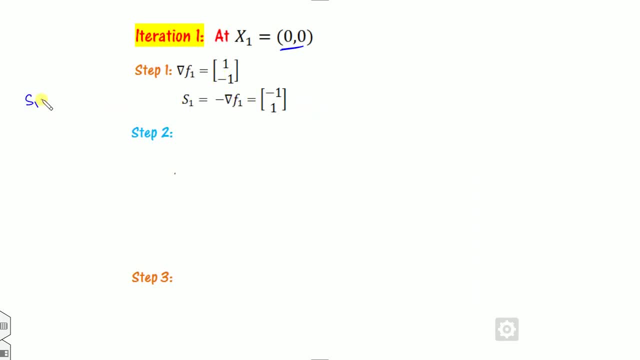 of the s1 is minus of the. so look at that. what is the value of the? s1 is minus this, plus beta 1, s0. and since the value of the s1 is 0, so it means the s1 is nothing but the minus. 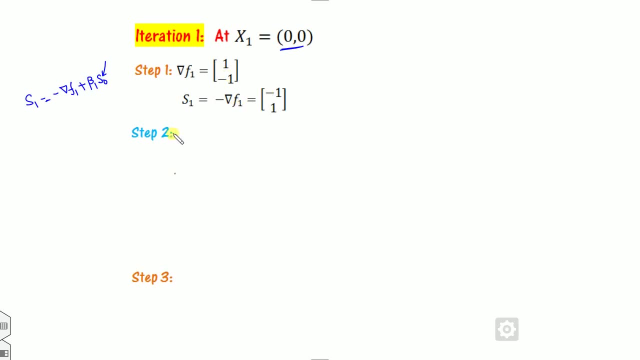 del f, 1. so this step 2 is calculate the value of the lambda. what is the value of the lambda is here. so what is the value of this gradient of transpose minus 1, 1? and here is minus 1, 1 divided by s1. 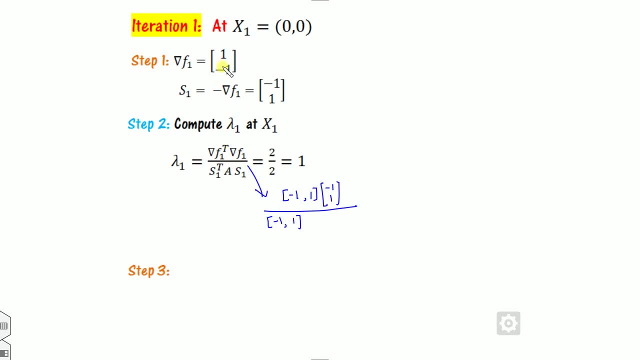 transpose: this is minus 1. sorry, this is a gradient. so this is plus 1, minus 1, and what is a is my look at the previous one case is this: what is s1 is my minus 1. so what is that? upside is 1 plus 1, and look at that, the below and this. 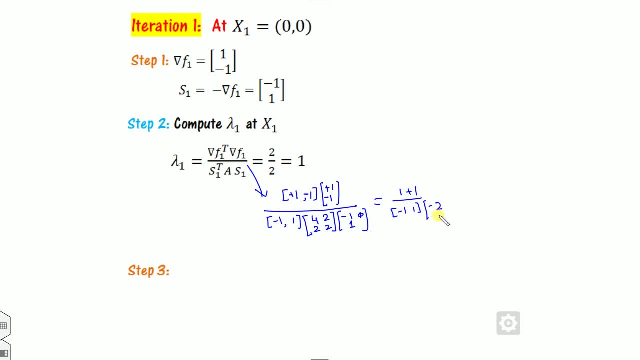 is my 1, this is minus 2 and this is my 0. so what is the value of? here is 2 and this is nothing but 91. now, after calculated as a lambda, 1, calculate the new point. x2 is nothing but x1 from the shown, so x1. 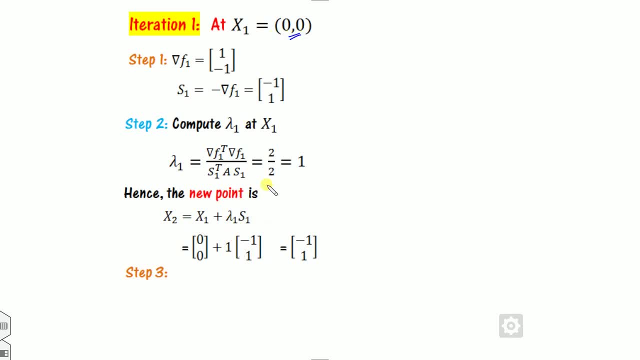 monsieur bangestliśmy, pointl a, que.2and let say with 1.x2 onto lambda 1. the new point, us Rem'x1pmx extra on, finds 60% of what is s 0, 0 lambda is my 1, s1 is here, so you will get this. check whether this point is optimal or not. 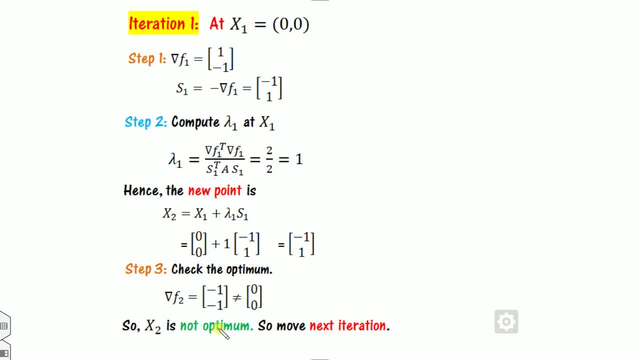 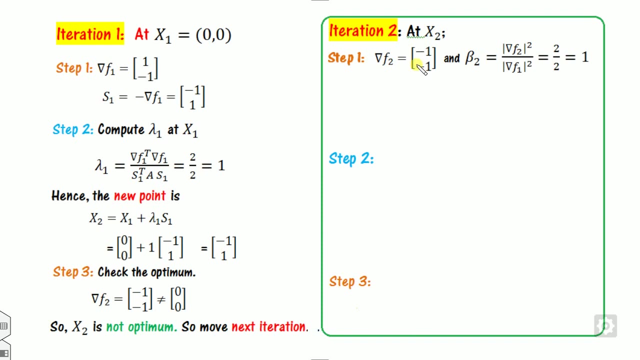 you can find the gradient value at this point. it is not 0, so it means we have to move this next step now, since we are using the conjugate gradient method and the n is my 2, so it means this step must be optimal. is there now? add the x2 again, calculate the del f2, so we have already. 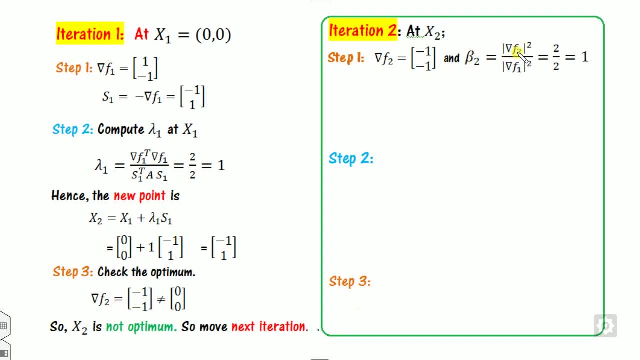 calculated that minus 1, 2, calculate the beta 2 gradient of 2: 3. so what is that? this is 1 square plus 1 square. how you find this is: this is nothing but this plus this, so it will be 2. what is the? 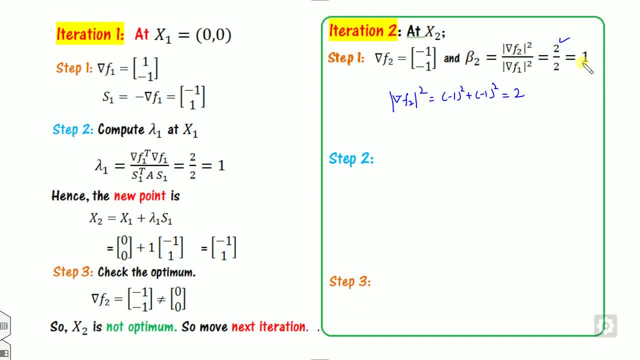 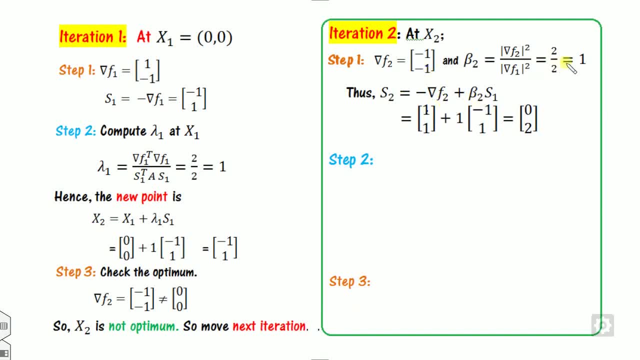 gradient 1 square is. look at the 1 square plus minus 1 square again. so you will hear. now calculate: the s2 is minus of this. minus of gradient is here. beta 2 is my 1 s1 i already calculated here. you will get 0- 2. now calculate the step 2, that is, calculate the value of the lambda. 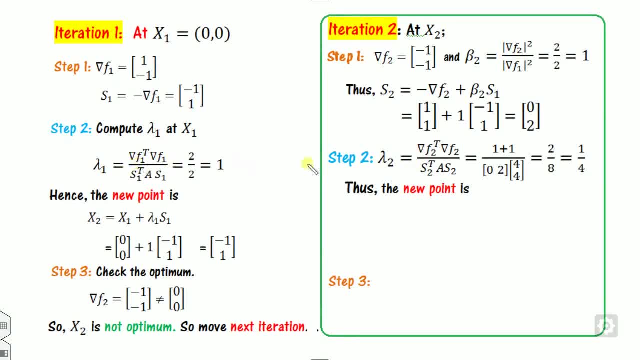 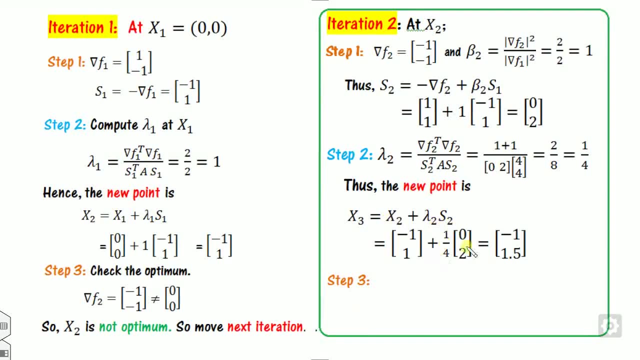 so lambda is. look at that. here is 1 index. is there? now it is 2. so you will get gradient of this. you will get 1 by 4. calculate the new point. here is x2. now you will get the x3. look at that. x3 is nothing but x2 plus lambda 2, s2. you will get this. check whether this point. 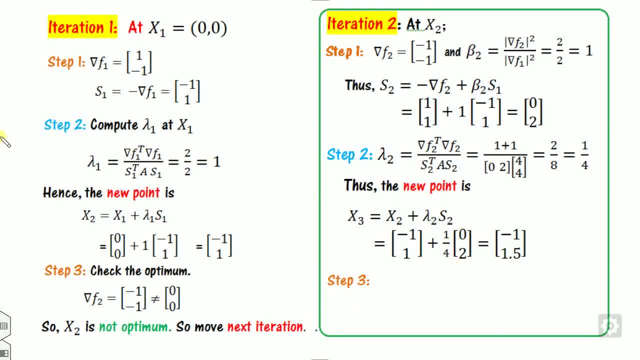 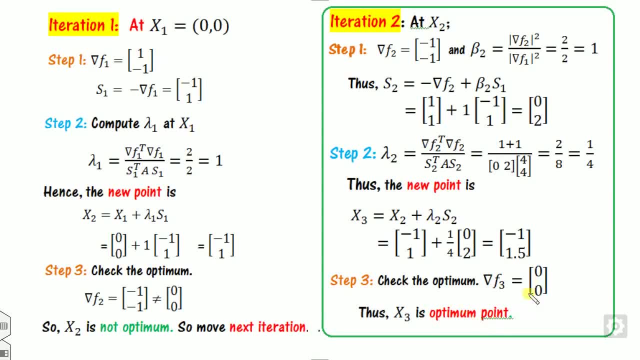 is optimal or not. and it must be optimal because we use the conjugate gradient and you can see that gradient will be 0. so it means the gradient is 0, it means the optimal point is reached. so this point is my optimal. so what is the answer? is x1 is my minus 1, x2 is my. 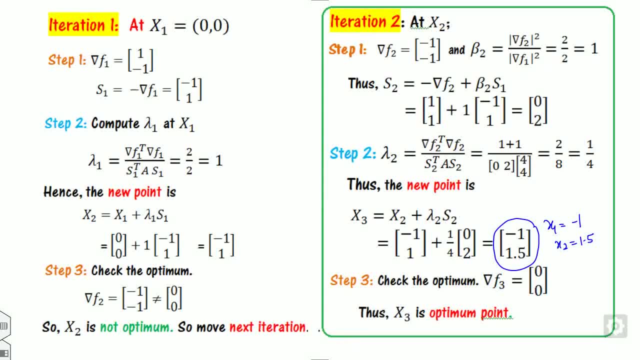 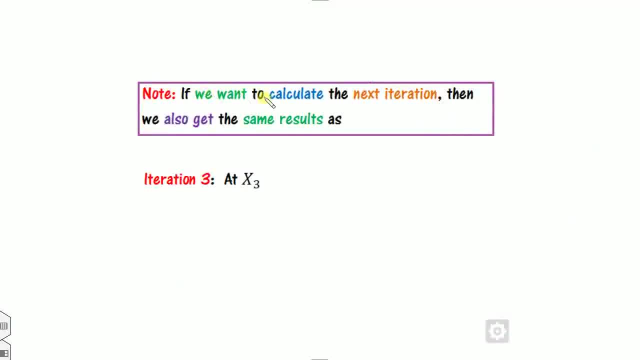 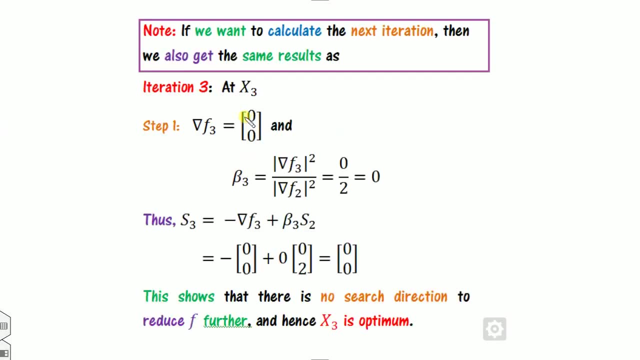 minus 1 plus 1 point. if you are still unable to remember that, the conjugate gradient will converge in at most end point. so what will you do? if you calculate the next situation, then it will also converges to the same point. If you calculate the gradient at x3, so you will get 0. calculate the beta 2, beta 3: it. 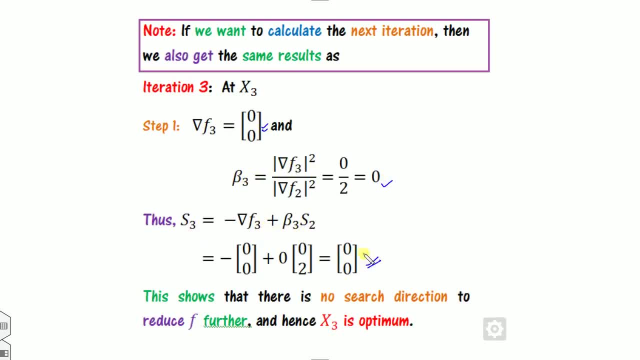 will be 0. so s3 is here. so look at the step 1. the gradient s is 0. it means there is no search direction to reduce further. it means x3 is my optimal. so I hope you can enjoy this session also and able to understand this conjugate gradient method for the more practice you 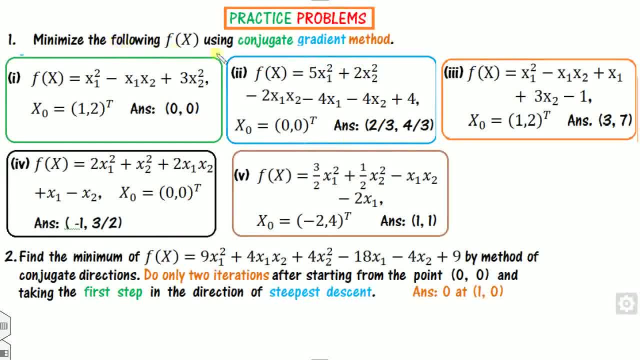 can solve this. 6 problems are there. solve them in conjugate gradient method. So here is a two decision variable. so optimal will reach at the most two steps, and so on. so you can try to solve these problems. if there is any doubt, you can ask me at any time.